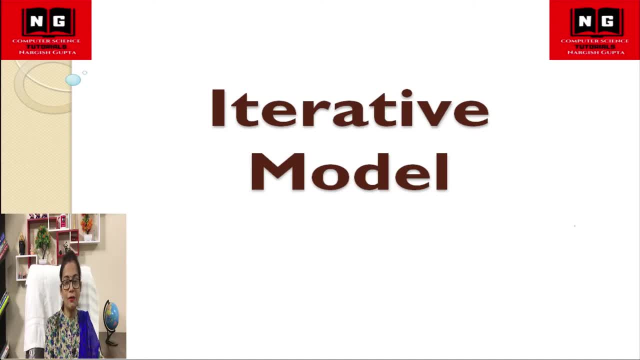 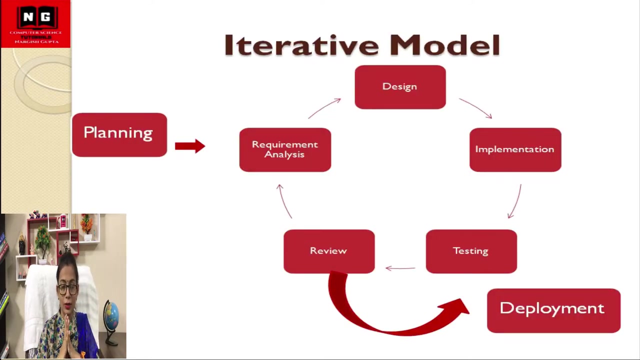 So let's start with the iterative model. As the name suggests, iterative means there will be iterations. Iterations means there will be a repetition of particular stages. as the name suggests, Let's see the model, or diagram, for iterative model. We can see the diagram over: 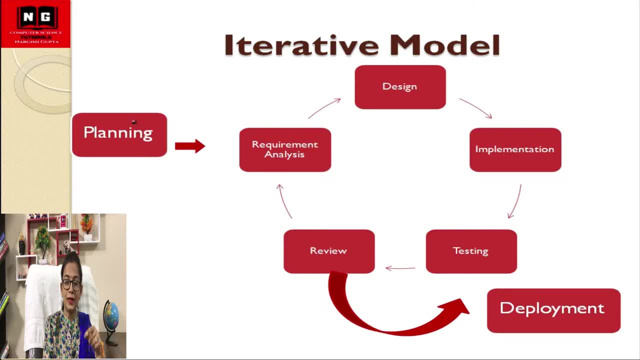 here The phases are almost same. There are planning, requirement analysis, design, implementation, testing review and deployment. Review is the added one. We will discuss it in this video. So, starting with the planning As the SDLC model, what we do in planning? We decide the feasibility of the 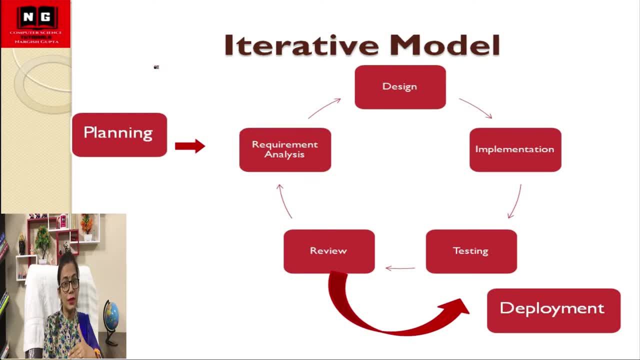 project that has come to us, What are the risks of it And can we move forward with that project or not? So these things are important. We decide all these things in the planning phase After planning. in planning we also decide that what kind of model we are going to adopt. So in planning we have decided all these things. 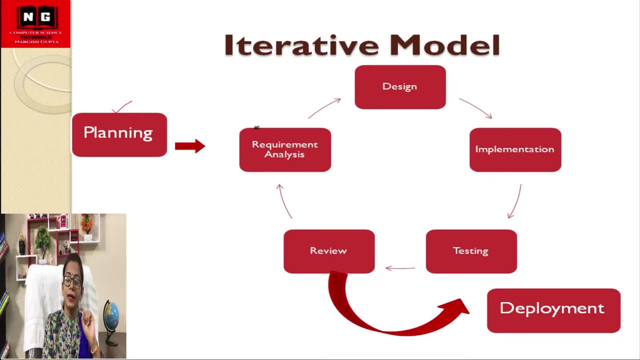 that, finally, we are going with the iterative model. What is the point of iterative model here? After planning, what comes first? Requirement analysis. What are we doing in requirement analysis? Whatever software we have given to the client, We will analyze the requirements of the client. What are the requirements? How are the expectations? 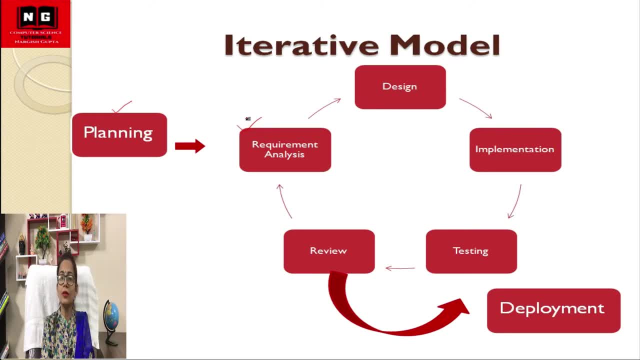 of the project that the client is telling us And how we have to compile it and make it. Then our next phase is design phase. In design phase, what we will do is we will deal with the designing of our project. How are we designing the project? And whatever software. 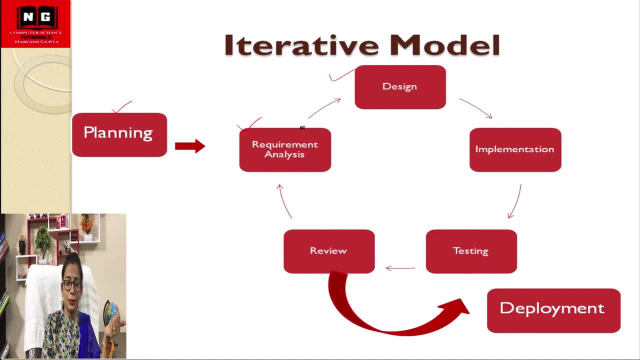 we have we do during the design phase. So, for example, in this project, as you have guys who have done apology to the client. So software is a very important thing that we have to do everything before we even design the project. after that we have to do everything. 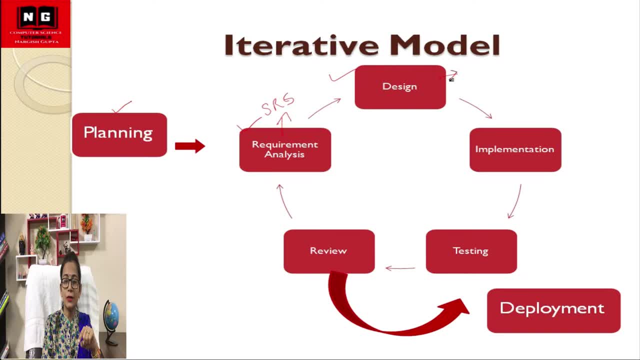 properly. Software requirement specification document. in our requirement analysis phase our software requirement specification document is developed. Okay, software requirement specification documents are developed. We use it as an input for the design phase and we also take our design document Which we get in the design document. according to that, we will implement the designs here by implementing. 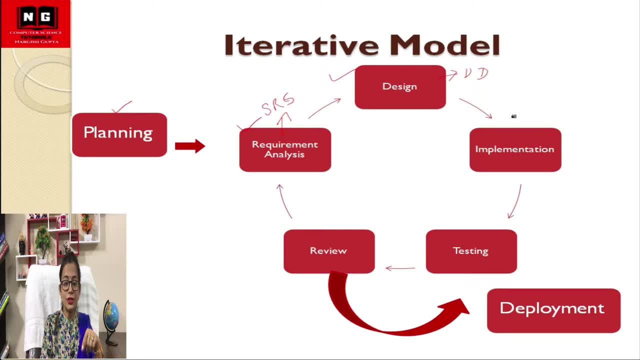 here. it Implements Implementation. It will get implemented. We are working through Apple department and we are working through this e-mail application. We also implement the design documents. Now, if you need this, we are going to implement for the� implementation ke. baat uski testing karein. Implementation kara, then implementation ke. 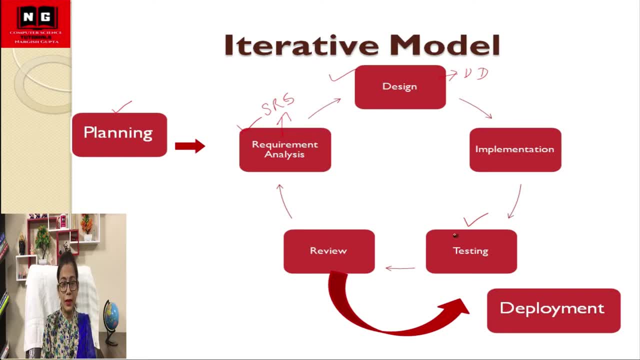 baat uski testing karein. Testing karne ke baat humare paas yaha pe ek extra phase aaya, that is review phase, which is the most important part of this iterative model. To hum is review phase mein. basically, kya kar rahe hain Jo bhi humne yaha pe requirement ko develop? 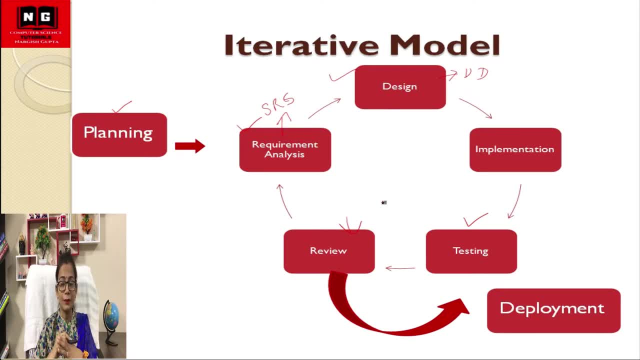 kara, usko customer se review karte hain To iterative model ka advantage. humara yahi hai ki iske andar hum pura jo software hota hai, uski development puri nahi karte hain. Ek specific part ko develop karte hain, aur usko review karate hain kise client se Client. 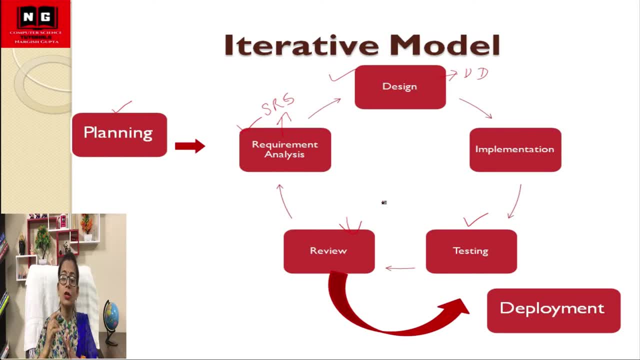 se review karane ke baat as per their feedback hum. dubara se review karane ke baat, as per feedback hum. Did you face issues before we used them In main area. there are lot of issues of quality, as well as quantity versus the quality of. 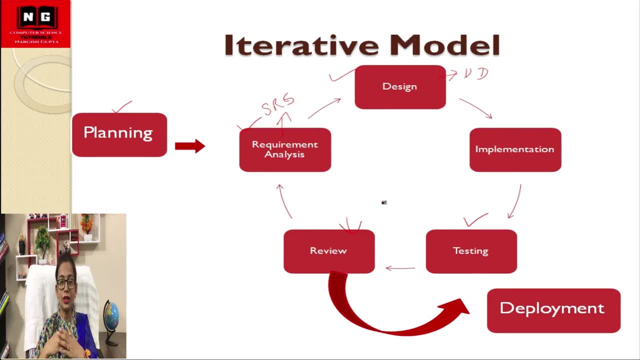 theemen And the quality and according to that feedback we move towards the next iteration and when these iterations are completed, after completing all these iterations, we go to deployment. so there can be two iterations, three iterations and multiple iterations. whatever the iteration is, after completion of iterations, we go to deployment. 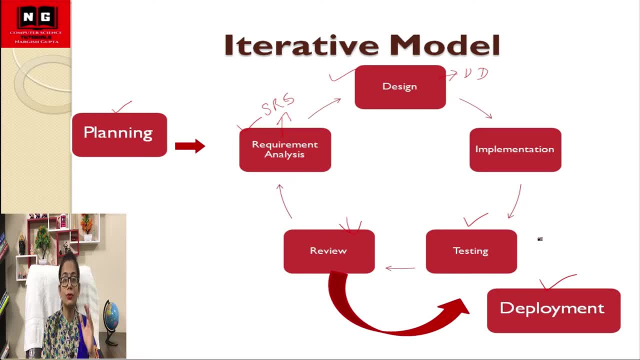 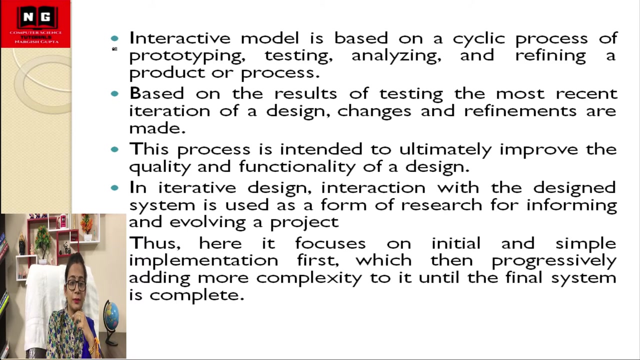 till then we only review our product or software from the client. so this is basically the process of our iterative model. in this we develop specific requirements of the project. let's see some basic points for iterative model over here. what are the basic points over here? what we can see is: 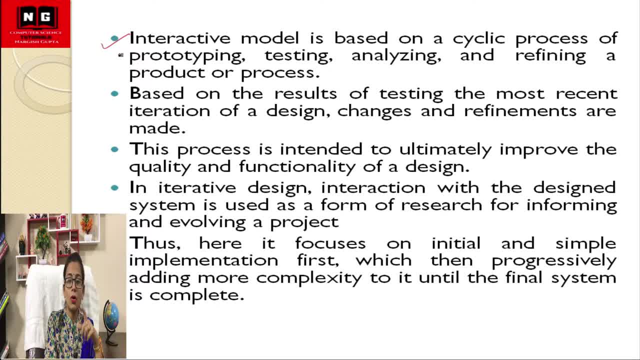 the iterative model is based on a cyclic process, the process of prototyping. so in waterfall model our drawback was that our customer or client was not able to see how the project will look. he used to see the project when it was completed. but by overcoming that drawback, what we introduced in the iterative model, 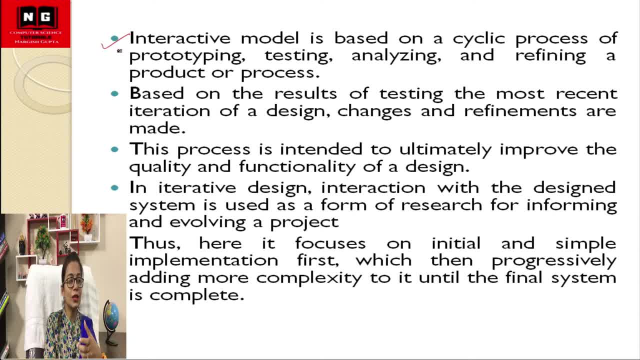 a process of prototyping. prototyping also means making a rough sketch of something, means suppose you are doing a painting, but before doing a painting you draw a sketch of it. so by drawing a sketch you show the client that, okay, the base of our painting will be like this: 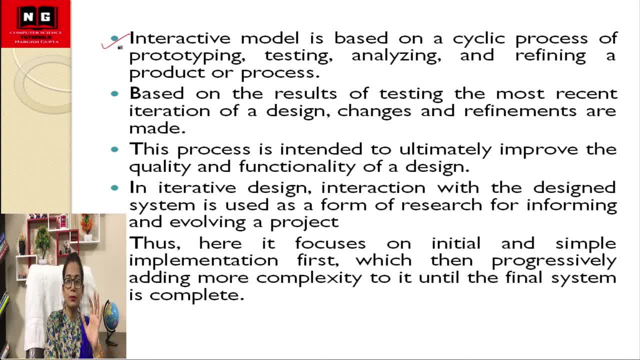 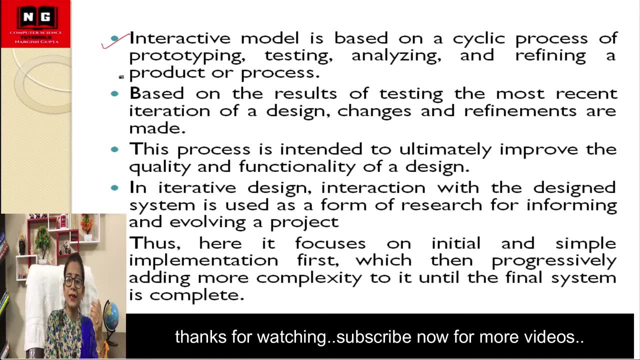 so the client also gets satisfied. okay, our product or software is being made. at the end it is going according to our expectation. so basically, what our iterative model does is there is a cyclic process and in that we are doing prototyping, testing, analyzing and refining a product or process. 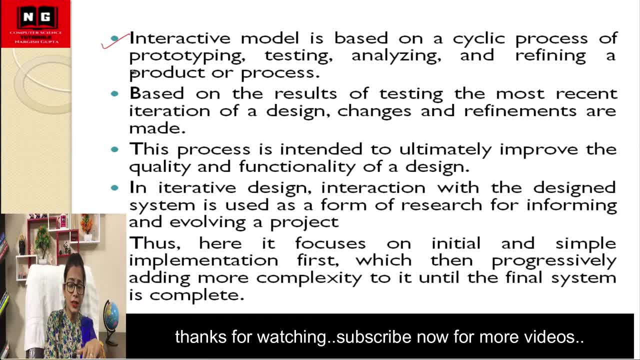 where is the refining part on our review now? the second point that we do refining is based on the results of testing. based on the results of testing, the most recent iteration means the result of the testing of the most recent iteration. according to that, we go to the next iteration. 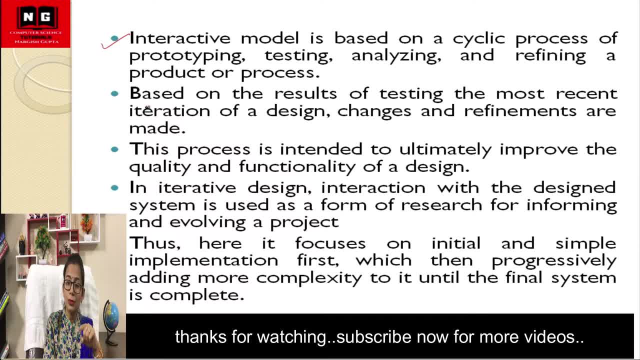 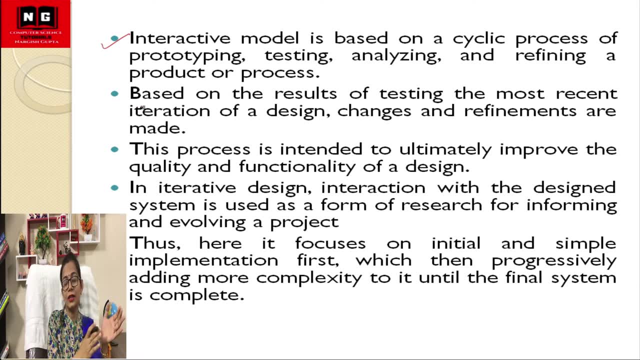 based on the result of testing the most recent iteration of the design, changes and refinement are made. so the changes and refinement that we bring in our project are based on the last iteration. suppose we are in the second iteration, so the feedback of the first iteration and the remaining requirements. 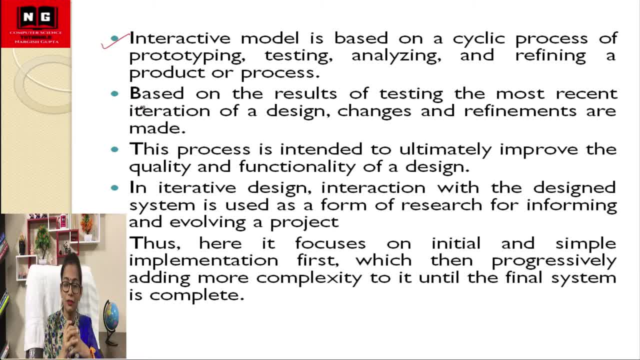 by involving both of them, we move towards the next iteration. now coming to the third point is: this process is intended to ultimately improve the quality and functionality of the design. it is a simple thing: when we are showing the client, the interaction of the client is proper. 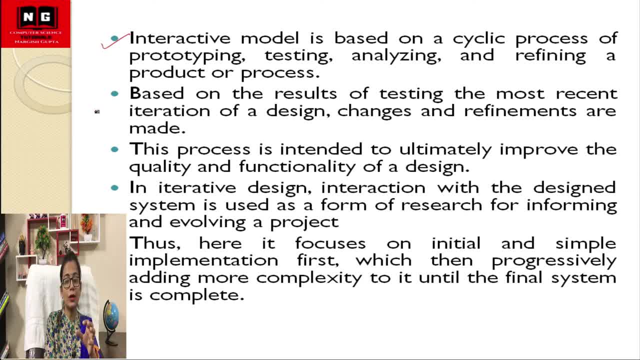 the client is reviewing, and again and again, the changes or the issues that are coming in the requirement. we are entertaining all of them. so thus this helps in the better quality of software delivery. now, coming to the fourth point. the fourth point is what our fourth point is telling us. 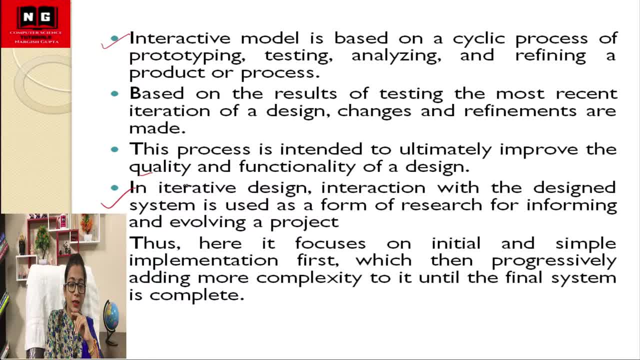 that what it is telling is, in iterative design, interaction with the designed system is used as a form of research for informing and evolving a project means what we are basically doing in this: in starting we are making a sketch of our software and then slowly, slowly, when we are adding things to it. 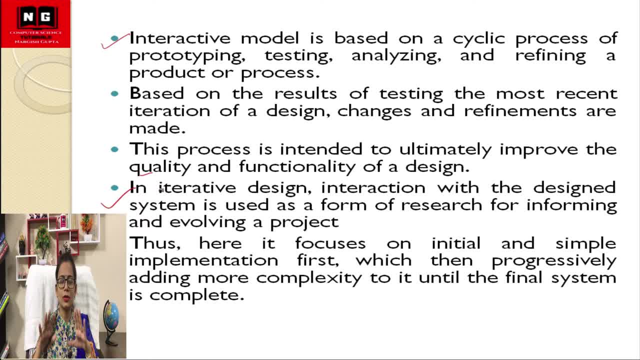 or in it. you can take it as a normal painting, that there is a painting in which you are drawing a mother and a daughter and there is a painting of them. so, first of all, we made a sketch. after making the sketch, after drawing the sketch, what we need to do in it. 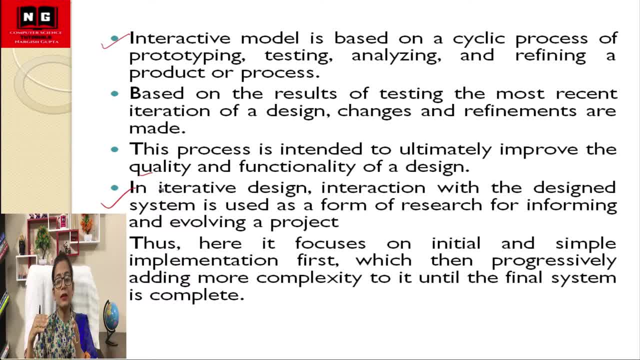 we need to fill the color. so the one color that we fill it is researched in a way. slowly, slowly we are enhancing it better and we are enhancing it so that basically helps to make our software more beautiful and to make it better helps. so iterative model helps us a lot in this. 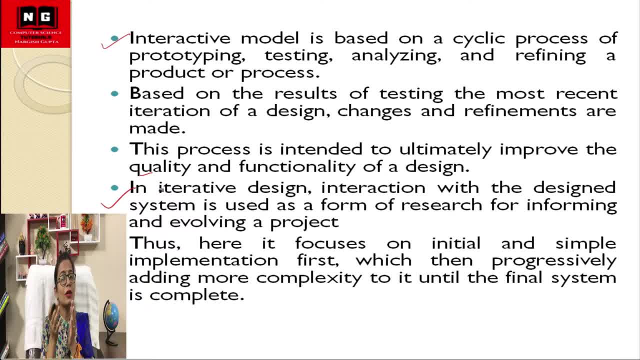 because we have got an overview, so we enhance it better. now, coming to the last point that is thus: here it focuses on initial and simple implementation. so here it is saying that here it focuses on initial and simple implementation first, which then progressively adding more complexity to it. 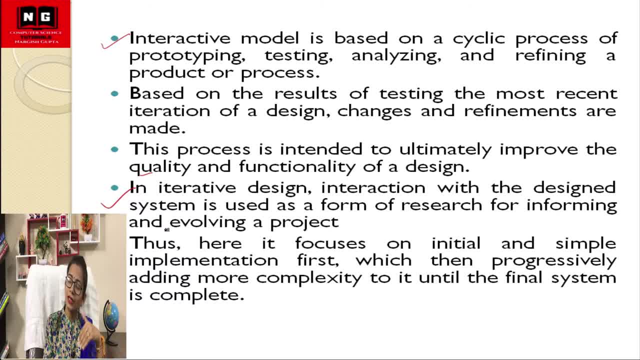 until the final system is complete. what we are trying to say here, that first we draw the simple things of our software and get it reviewed. then slowly, slowly, the simple things that we have made, the related complexities. we are adding them slowly. slowly means first a simple requirement. 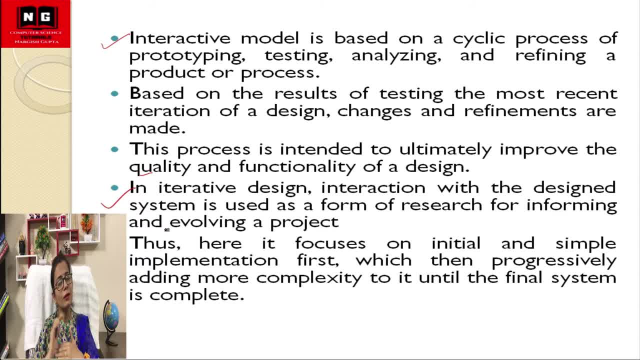 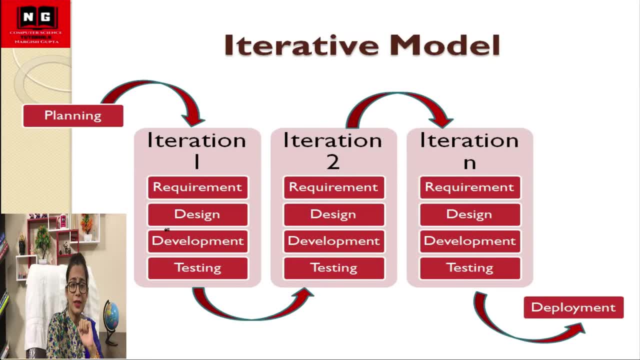 is covered, then we move towards complex requirements. these are some of our points related to iterative model. now I have again made a diagram for iterative model through which we deal with an example. we have got a project in which we have to make login registration page, login registration. 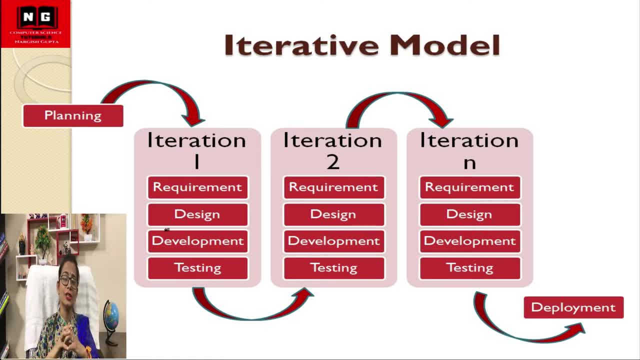 and a welcome page. we need these three pages and this client has given us its requirement. so, in planning, first of all, our client has told us that this is our so and so project. it is a login project and their login id is not there. they will register. 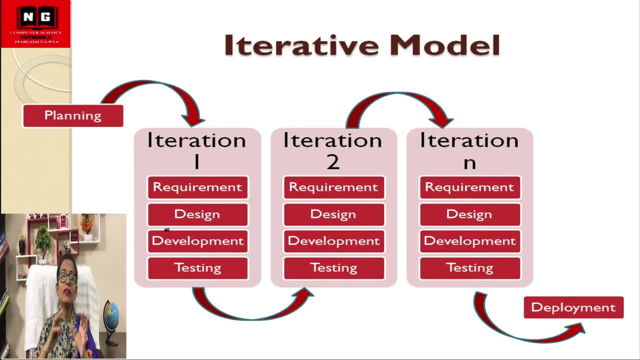 so our registration process will come and then a welcome page will come. so in this planning, we decided: ok, this is fine, it will work. now we will come to the next page. ok, we are using iterative model for this. now what happened? we have a lot of means. these are three pages. 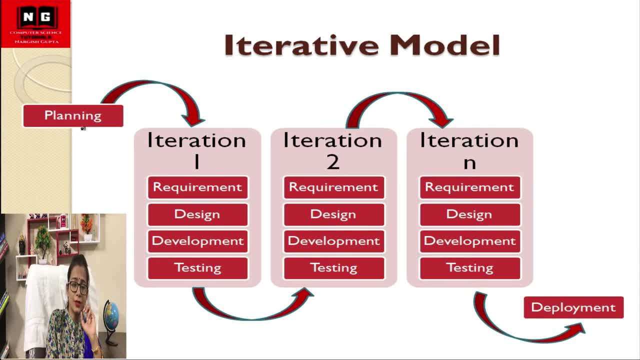 according to this, what we understand? that we have three pages, which are: one is login page, then one is registration page, then one is welcome page. ok, login page, registration page and welcome page. we have three pages. so first means, in iterative model, how we will do development, what we will do. 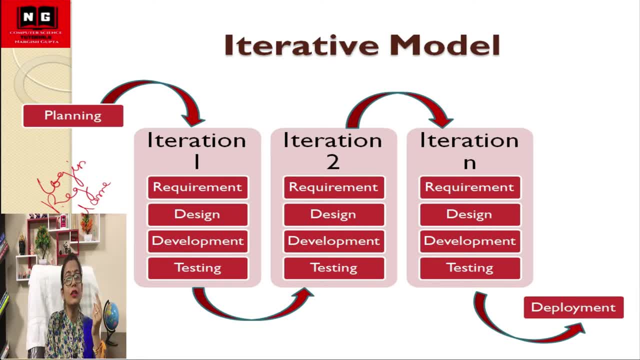 login, registration and welcome. we will make these three pages in first iteration but we will make a rough sketch. that what we did in login there will be two text boxes: username and password. we will put that in registration. we have given some particular fields. one we have made: wireframe. 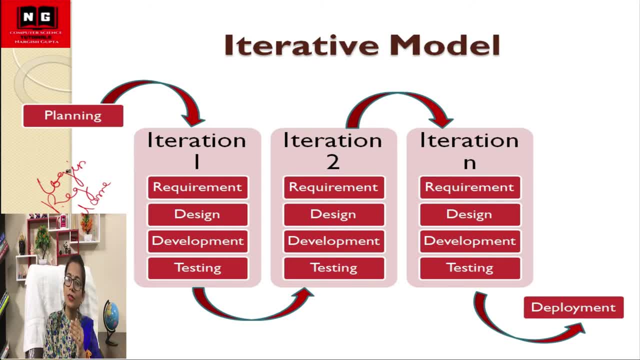 then we have made welcome page how it will look. we have developed these three pages individually, individually developed, in which, in first iteration, so according to our requirements, we have developed and we come to it and check it in the testing page, that brother, the login, according to all the requirements. 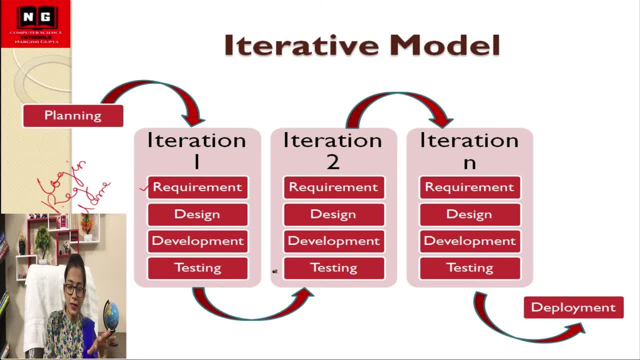 we have seen all these things are correct. ok, then, from here our second iteration. so, basically, what is happening at this place? our review is happening. so here what is happening in the review? now our customer will see that the way he wanted: login page, registration page and welcome page. 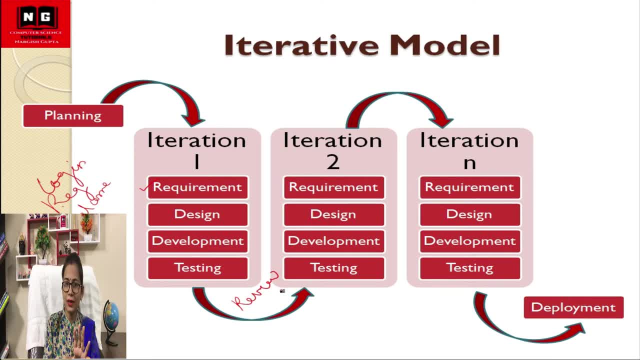 he wanted that. something looks like that. yes, it looks fine. now these three have no connectivity. then what we go to the next iteration, in the next iteration we have no other remaining requirements. what we saw in that, what we did in that login page, in that page we have 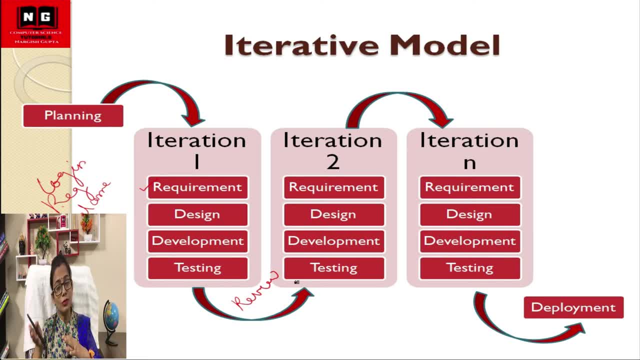 submit button. when we click, then we go to that page, welcome page, or if there is no id, then the registration page, the functionality we go to. that means add buttons, add their clicks in the second iteration and some validation should be applied. then you apply. that means simply. 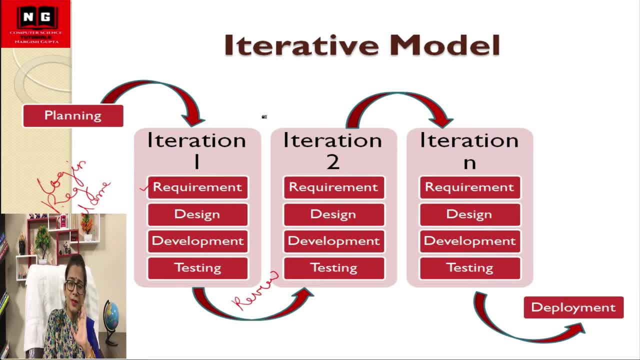 in the second iteration we have. basically, in the second iteration we have clicks here in the page we have button clicks involved, button clicks involved. ok, now, after that we come to the next iteration. next, here we have multiple iterations. that's why I have written an iteration. but now suppose 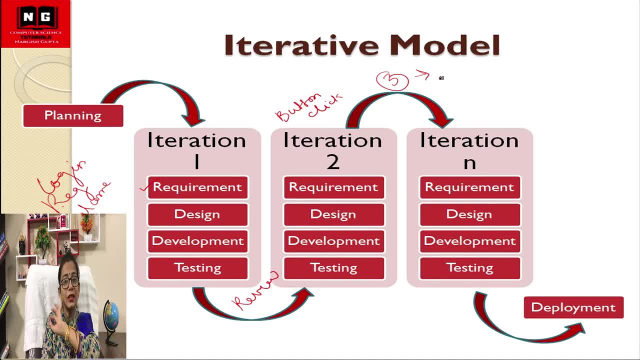 we go to the third iteration. what we did in the third iteration, we did the connectivity of the page, but it was that, whatever you put, we are able to go to that page. we have put the validation. ok, we have put the validation. the validation was left. login page. 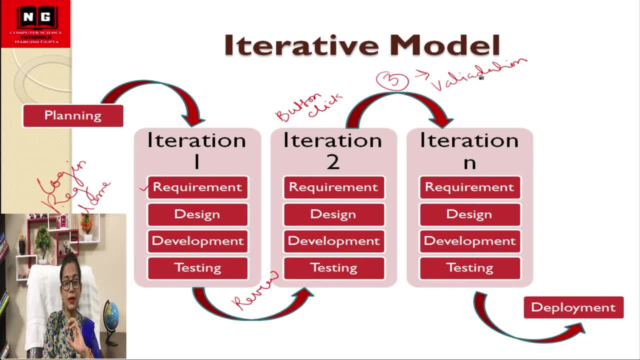 and registration page. we have put the validation of both the pages. this is our third iteration. then what we can do, we go to the fourth iteration. what will happen in the fourth iteration? the remaining requirements means, like the forgot password thing came and in registration some particular issue. 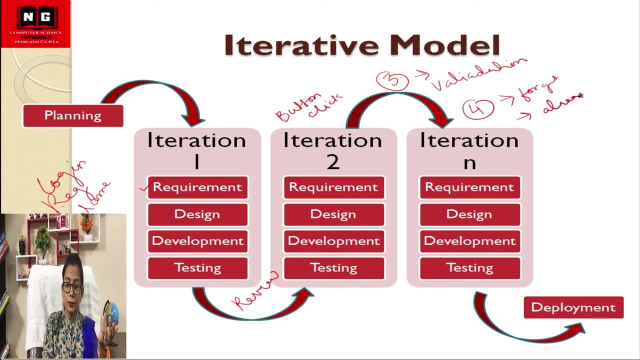 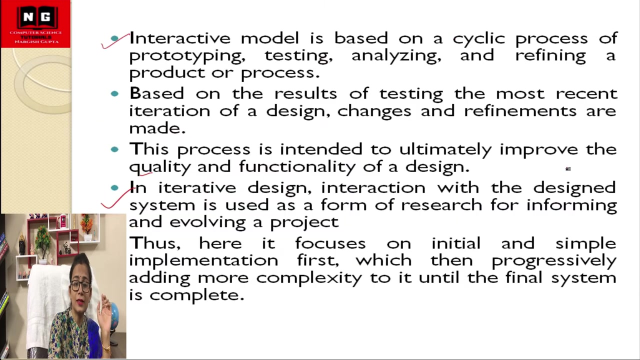 came or already registered, which already registered users. things are that kind of error handling we have done here. so our project we completed in four iterations and then we delivered it for deployment means what happened. we gave its delivery. so we saw this model last cycle and in between. 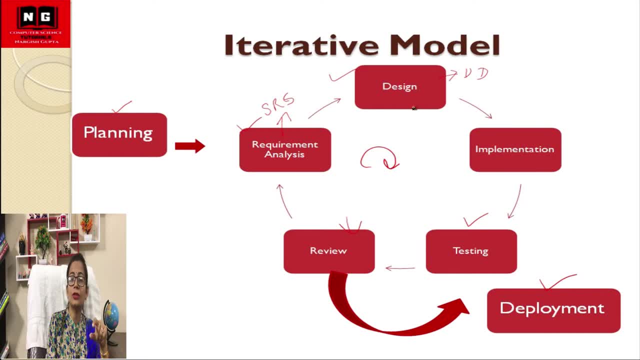 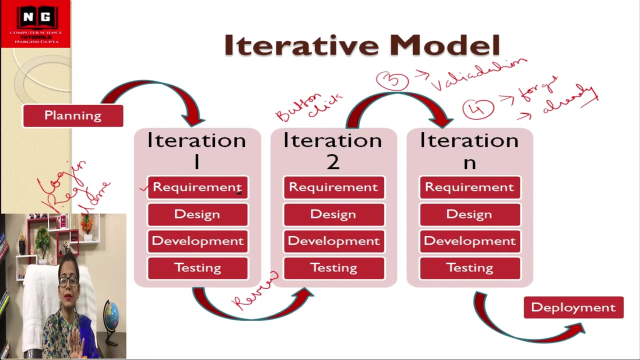 cycle is running. so this whole cycle, basically this whole cycle, it keeps repeating: until the customer is satisfied, we do not take its delivery. when our customer will be satisfied by the review, then its delivery will come, basically. so we have this thing here. this is the development. this is not. 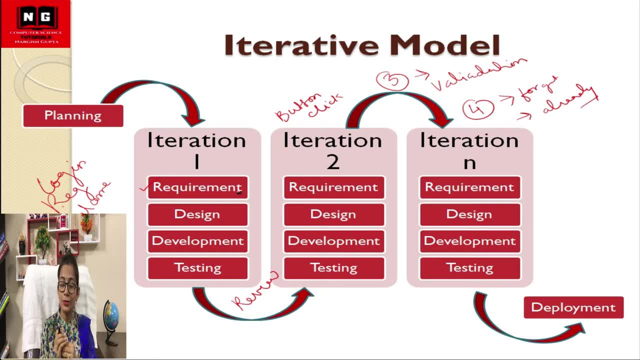 that we made login page one iteration, then another iteration. no, we are covering the whole project. we are not working on a particular part of the project, we are covering the whole project. but first we took simple functionality, then slowly we added more complex functionalities, then slowly we added: 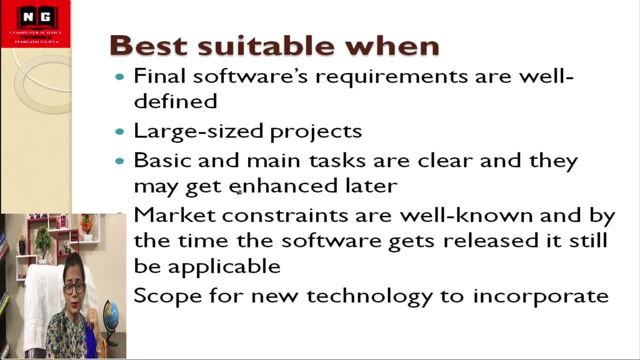 more complex functionalities. now let's come to the point. coming to this point, our first point: in those softwares or in those projects whose requirements are well defined, because in this also more requirement changes can be handled. but it is not that more requirement changes can be handled. 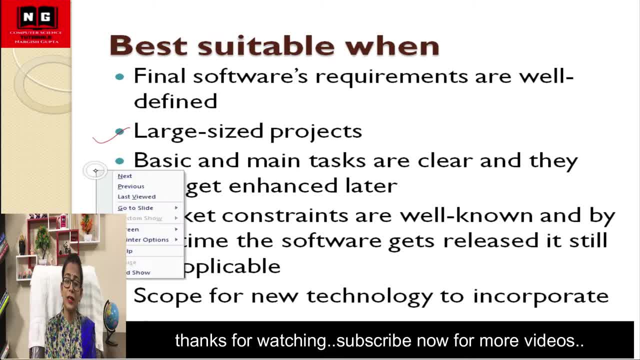 then it can be used in large size projects. now, third point: what is written? basic and main tasks. so we know basic tasks and main tasks means whatever tasks. we know our pages clearly. then we made a simple view which we discussed. then we enhance it slowly. we are doing. 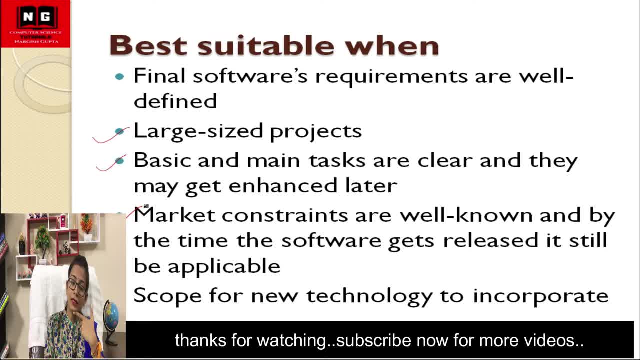 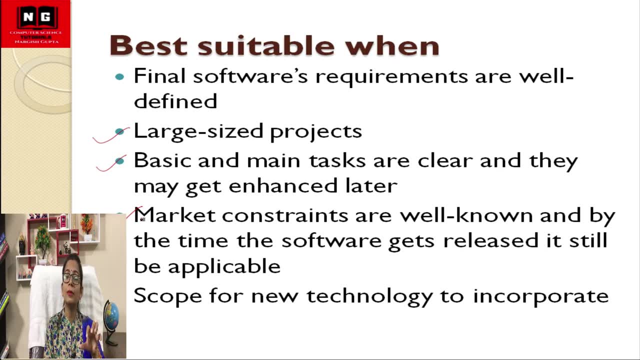 enhancement in this. then our fourth point is market constraints are well known and by the time our software will be released, then also our software will be applicable. how? because whatever changes come in the market, we are ready to handle it through this model. thus iterative model is getting 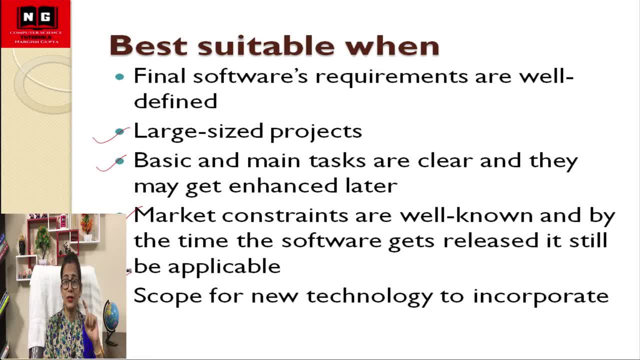 very useful for us. now. last point, which is the main point here: that scope of new technology to incorporate means we have to make that project on some new technology. so iterative model is a good point or good model to use, because initially you are starting to use some new. 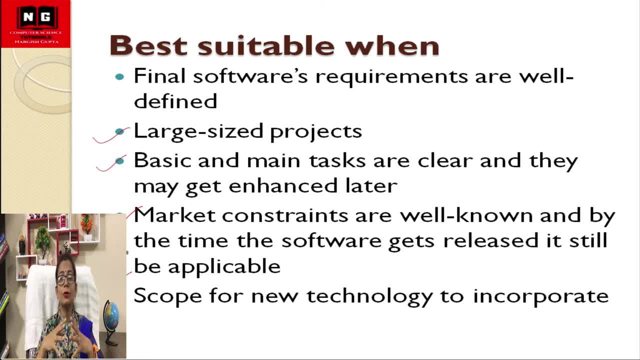 technology then there can be many problems, risks can be developed or not. so that thing we will know in starting in first iteration. this is a big point. suppose we went to first iteration and after going to first iteration customer says whatever project we gave it is not matching. 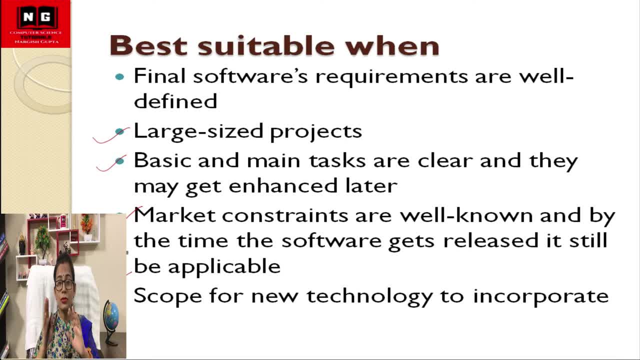 so we cross that iteration means the software or the prototype will be discarded. then we will start iteration again. there will not be any problem if we use that technology and suppose, with that technology we will get idea in first iteration that we can move forward or not. so if we 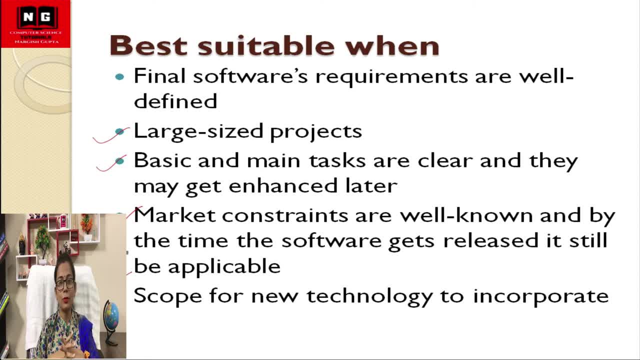 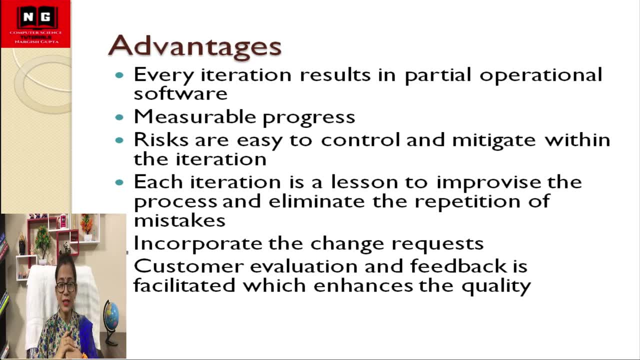 cannot move, then we can discard it. so our time goes and proper management goes. now coming to the pros and cons, or advantages and disadvantages, of iterative software. every iteration results in the partial operational software. so what is CBC? what is happening? in every iteration we are getting a partial. 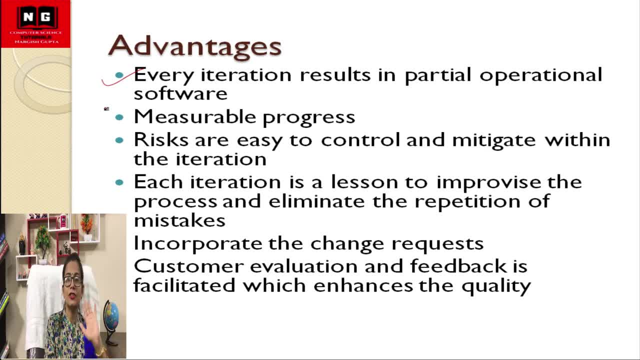 operational software. ok, because we have given three parts with different examples. we are getting a partial software, next measurable, and at the end we get to know what is the progress. that progress is going well or not. we get to know at the end now what is measurable, how. 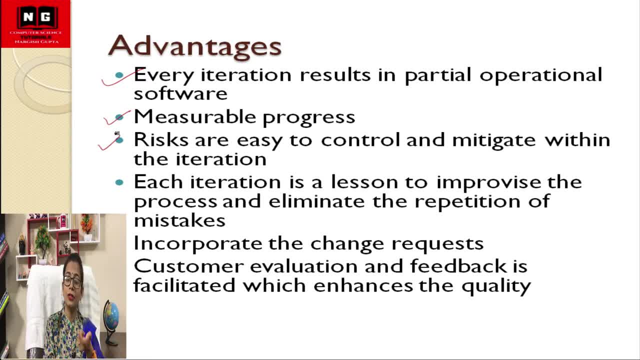 because again and again we are reviewing that thing. now, coming to the third point, that is, risk are easy to control and mitigate within the iteration risk. we can mitigate, see and analyze each iteration, the process and eliminate the repetition of mistakes. what is the advantage of this? the best thing? 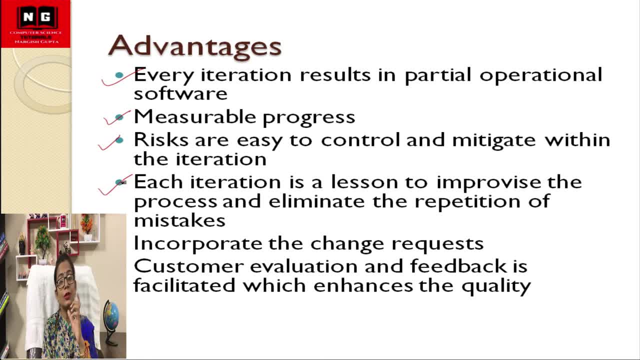 that is happening is that we are improving our product or our software in every iteration. we are improving it, we are enhancing it in every iteration, and the flaws are being discarded gradually. so this is an advantage for us, and thus it leads to the development of quality software. 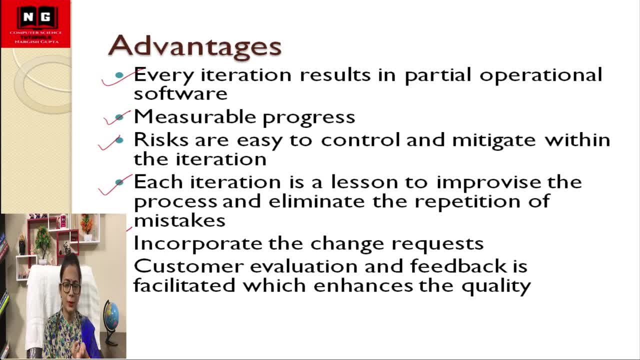 then this point is in corporate change requirements. it is helping us, we can take change requirements. then, last point comes: that key customer evaluation and feedback is facilitated, which enhances the quality, same point that we are able to review from the customer, so we are able to increase the quality. 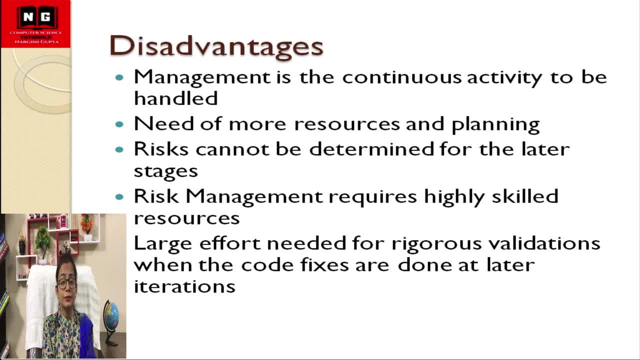 now coming to the disadvantages of iterative model. what are the disadvantages? management is continuously active means here the role of management is very big. so the management of our project should be so active that it continuously monitors that thing, because if there is nothing lacking from management, then that will lead. 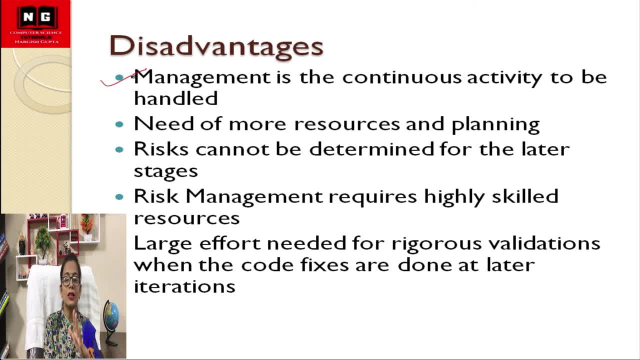 to the dissatisfaction of the customer. so management has to be continuously active. then needs of more resources. iteration can be repeated again and again. new resources can be needed and proper planning is needed now risk- risk cannot be. risk cannot be determined for the later stages. in starting we are analyzing. 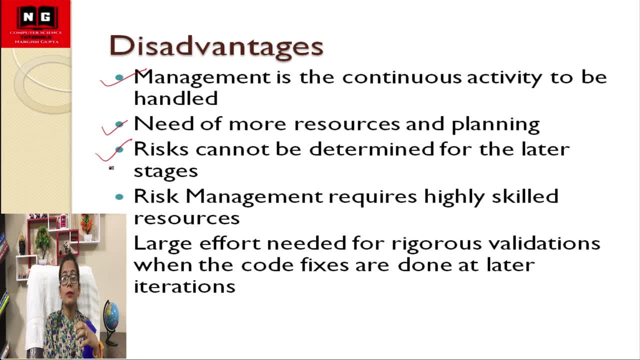 risk in every iteration, but many times there can be such chances that at the end, when we integrate things, then higher risk can come. so management requires highly skilled resources. so whatever people are involved in risk management, they should be so skilled that they should analyze the risk properly. 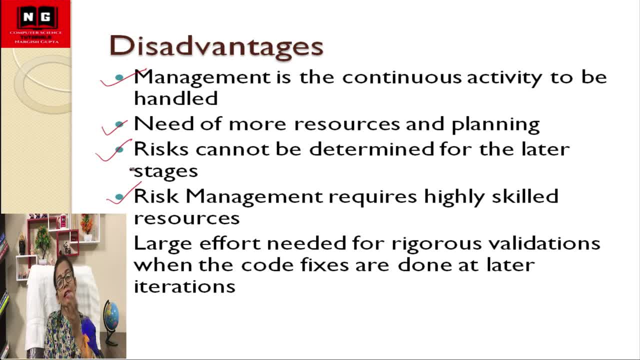 this is the biggest disadvantage: if we don't analyze it, then it will not start, and we saw this in the last video: that if any risk or any issue we get at the end of the project, now coming to the last point, that is, last point of our